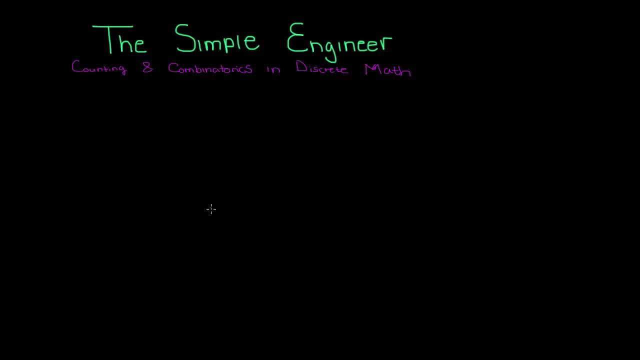 specifically designed for discrete mathematics. So we'll go through a few examples and we'll explain how these examples are done and hopefully you have a better understanding of some of the rules used in combinatorics. So, first off, our first example deals with different ways to 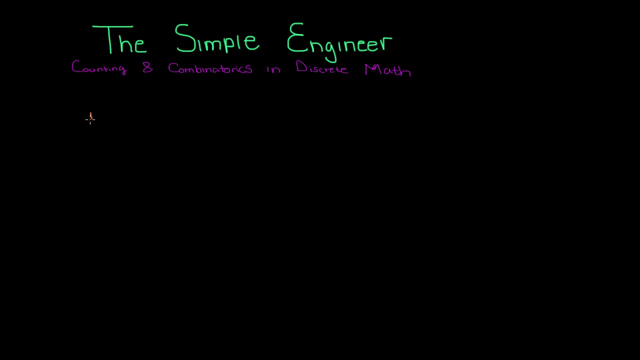 achieve a certain outcome. So the example goes by. there's a guy on the beach and he's selling ice cream from the boardwalk. He has three flavors: He has vanilla, he has chocolate, he has strawberry, blueberry and pistachio. 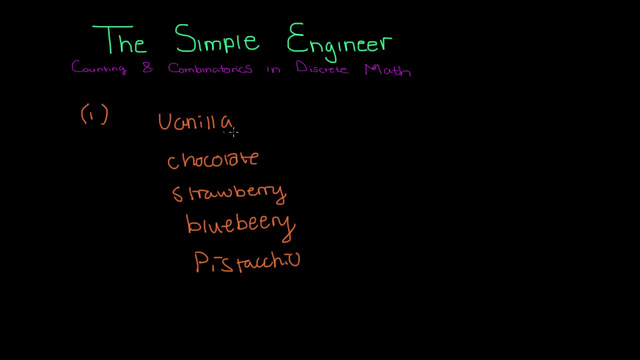 Okay, now these different flavors can either be served in a waffle cone, we have a sugar cone and we have just a regular cone. So the question asks: how many different single scoop ice cream cones can you buy from this guy? Well, you can look at this and say, oh, I can have vanilla with. 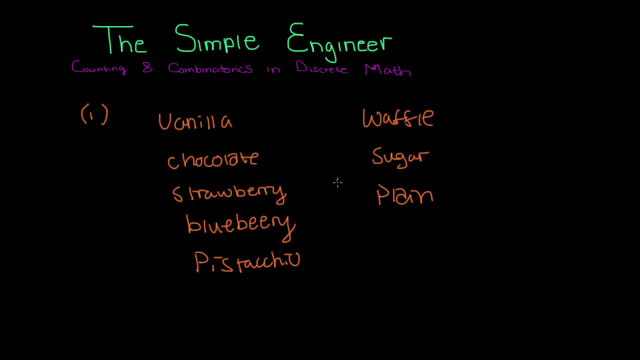 waffle, vanilla with sugar, vanilla with plain chocolate, blah, blah, blah, etc. etc. But there's an idea that goes along with these types of problems and it's known as the product, The product rule And what the product rule says. if there are in-one ways to do the first task and in-two, 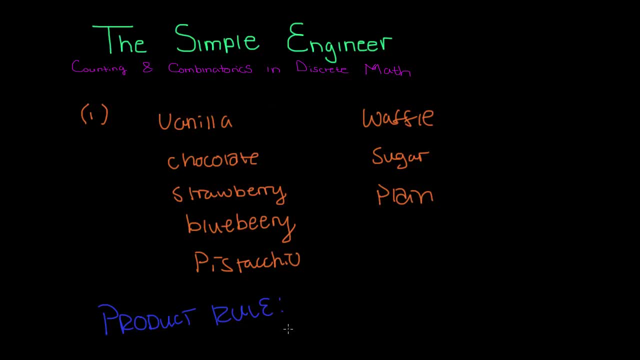 ways to do the second task. then there are in-one times, in-two ways to do the entire procedure. So our procedure in this case is: how many different single scoop ice cream cone combinations can we have from this guy? So this would be our in-one task and this would be our in- suic decided And the score have to belong to which idea a lot of them are like Pe consolidated, And usually it's either or multiple, just like combine them on one, or like save multiple, not just share. So we're just going to call it a formula. So it'll be a formula to do is take the extra two to oneипolar, Then we're going. 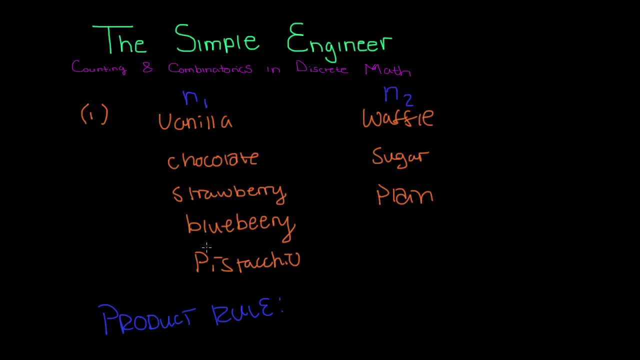 this would be our in two tasks. So there's in one flavors within two waffle cones. So here we have three types of cones, three types of cones, And here we have how many flavors. we have three, four, five types of flavors. Therefore, by the product rule, five times three, we would have. 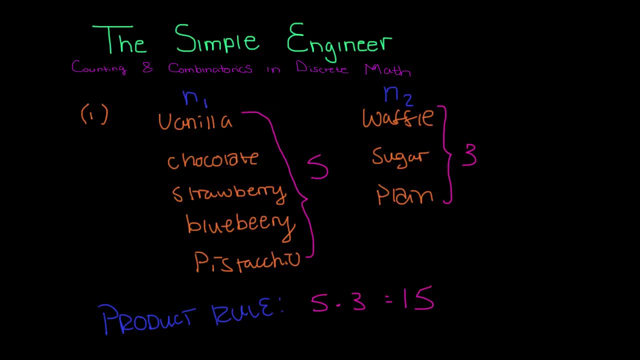 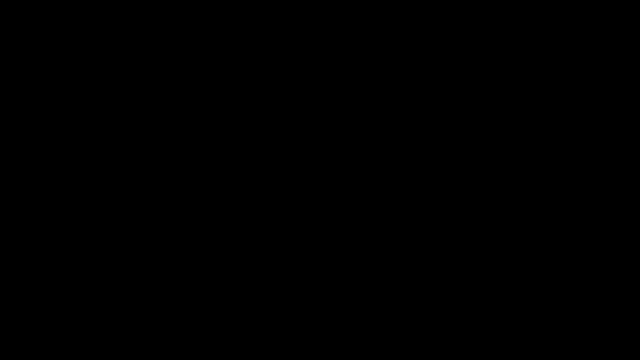 15 different choices. So that's how we do that first type of problem. Now let's go ahead and move on to example two. This one is a little trickier but still follows a similar idea. This is a license plate problem. So problem two says that we have a license plate and it can. 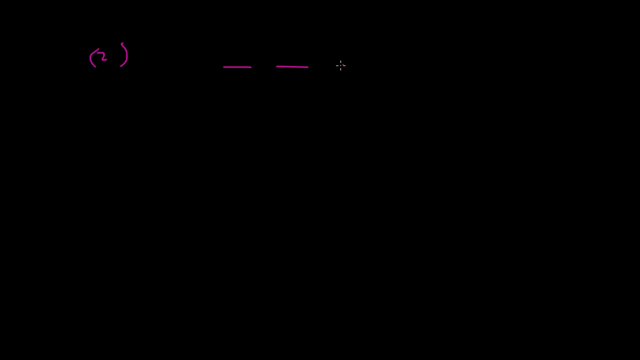 display two digits, followed by three letters, followed by another two digits. So here we'll label: we have a digit, a digit, we have a letter letter, letter digit and a digit. So how many different standard license plates are possible in this? 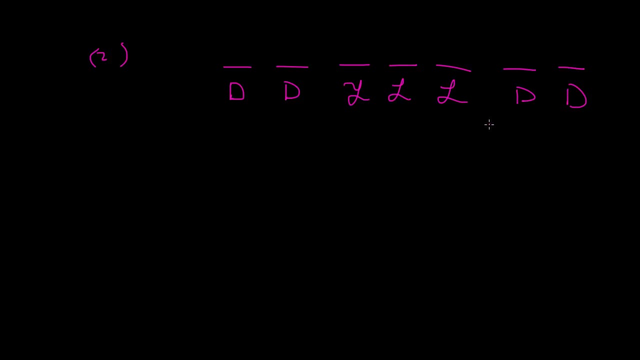 system. So we're going to assume that the repetition of letters and digits is allowed. So in digits, counting in base 10, you know that we have zero through nine, which is 10.. So we have 10 choices here. 10 choices here because repetition is allowed. Then for letters: 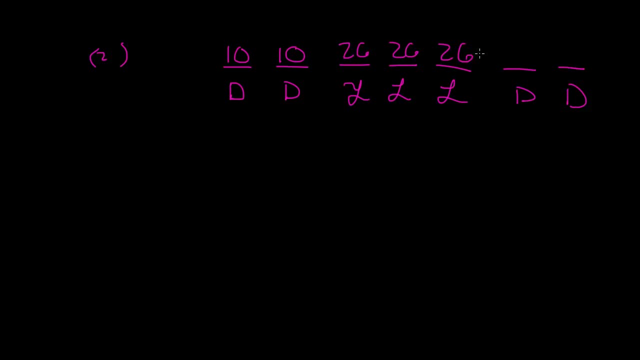 you know that there's 26 letters in the standard English alphabet and 10 and 10.. So, once again, we're going to have to multiply this by the product rule. Since there are, in one ways to do this and into two ways to do another, tasks, digits and letters, we would just multiply them out. So 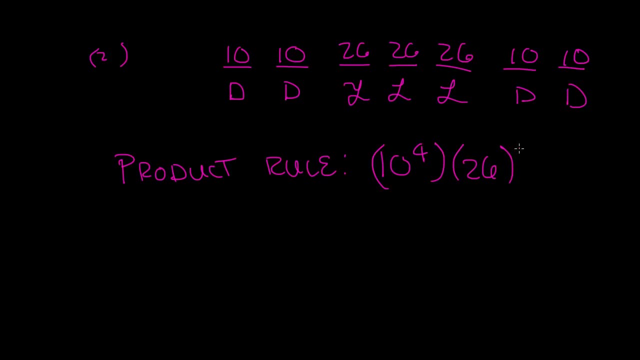 simplify, this is 10 to the fourth times 26 cubed, And what you end up coming out with as a final answer should be 175760000.. So the other thing we're going to have to do is multiply this by the product rule. So we're going to have to multiply this by the product rule. So 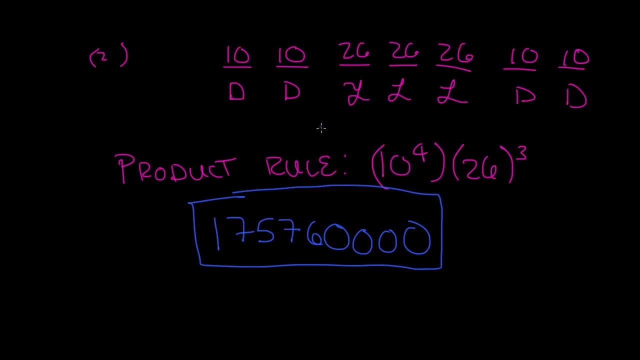 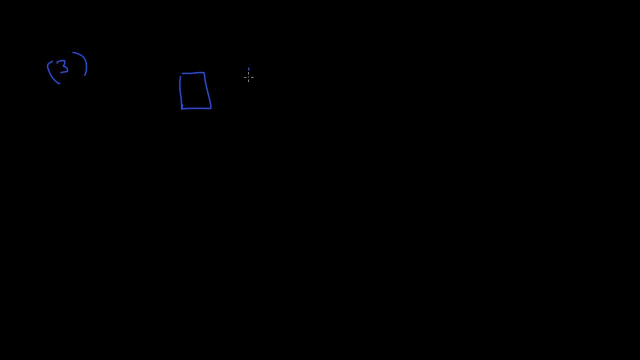 And these are the possible combinations of having a license plate following this standard. Okay, let's go ahead and move on to the next example here. Okay, so here example three. Okay, so we have four different dice. You know that each dice, each die, has six possible numbers on it. 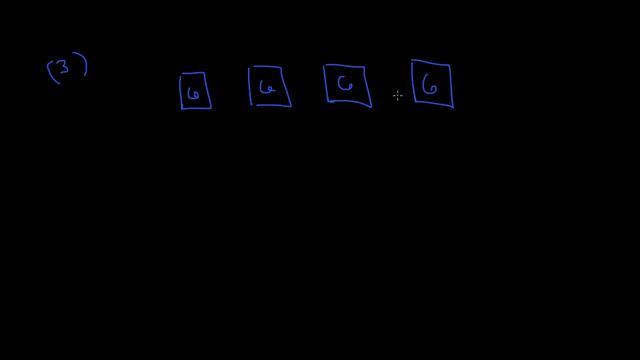 And the number of each die is recorded as you roll them. So they want to know how many different outcomes are possible with these four different die. Well, you know that six here times six here, times six here times six here would be six To the fourth, which equals 1,296 combinations. 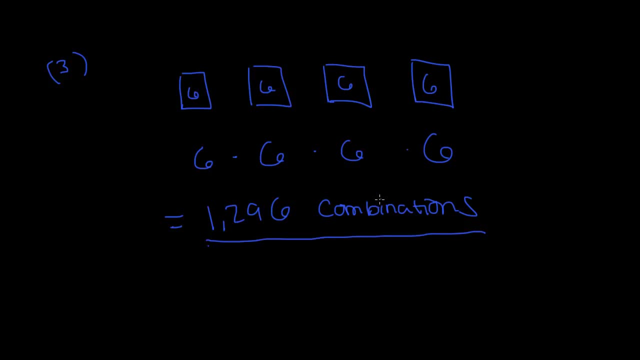 Assuming repetition is a lot. That's what combinations are. Okay, so not too bad. not too bad. We'll go ahead and move on to a couple more complex examples. Let's go ahead and look at how true and false are recorded. 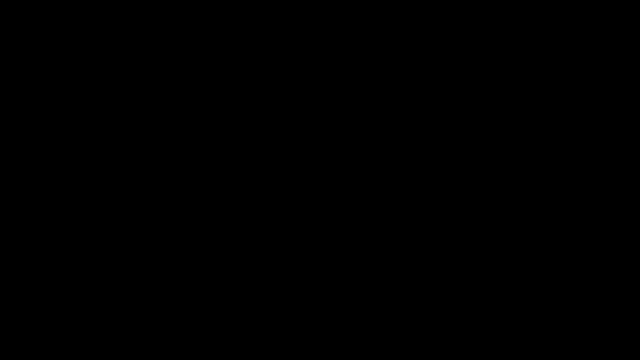 This kind of deals with how exponentials are treated And counting and combinatorics. So say that you have a true and false test that contains 12 questions On this test. it wants to know how many different ways can the 12-question test be answered. 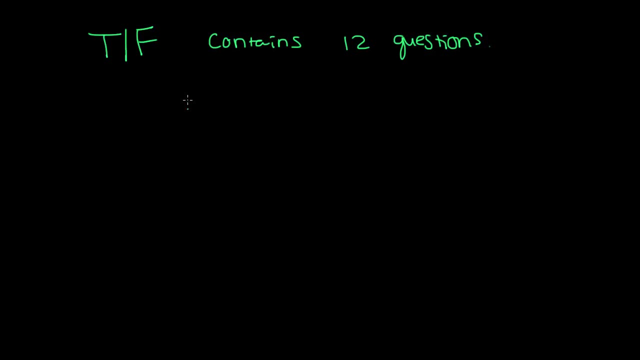 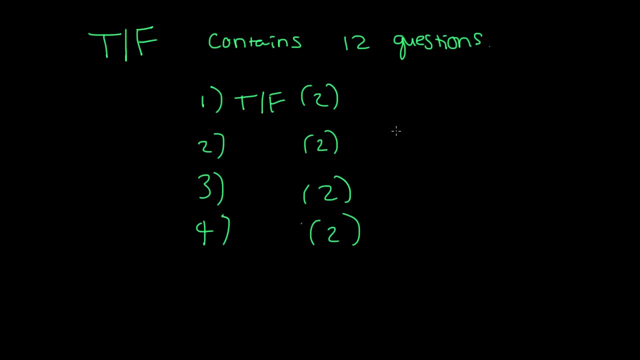 and all the way to 12.. So just looking at it from this standpoint, from like a diagram, you can see that two to the 12 is the answer, because there's two possible answers for each question. There's 12 questions: Two to the 12.. 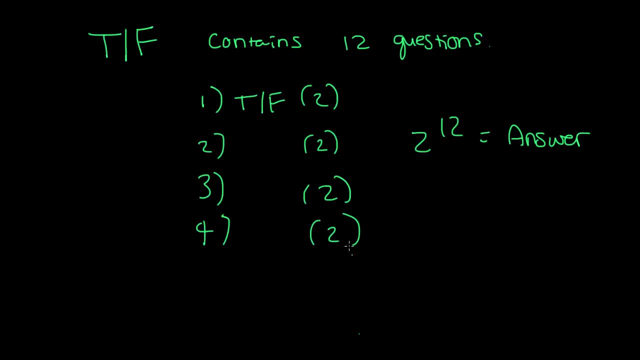 And this would equal 4,000.. So that would equal 4,096 possible choices. Okay, Moving right along, we'll do a couple more examples and hopefully you guys start to understand the idea of counting in discrete. Go ahead and get a new slot here. 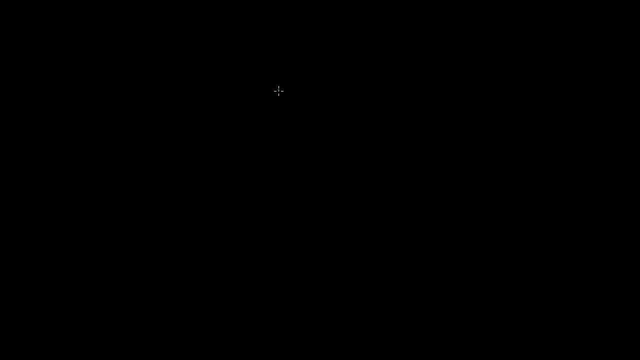 Okay. so the next question I'll ask you guys refers to digit combinations. So say, we have a three-digit number, okay, But this digit is formed using only the numbers one, two, three, four, five, six and seven. 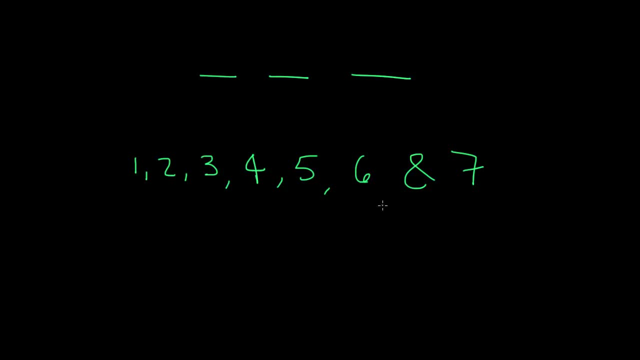 And they want to know how many different three-digit number combinations can be formed with repetition. So repetition is allowed. So if you go ahead and count The number of digits listed, you see we have one, two, three, four, five, six, seven. okay. 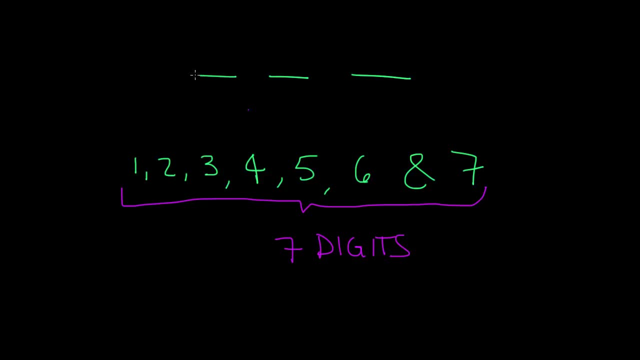 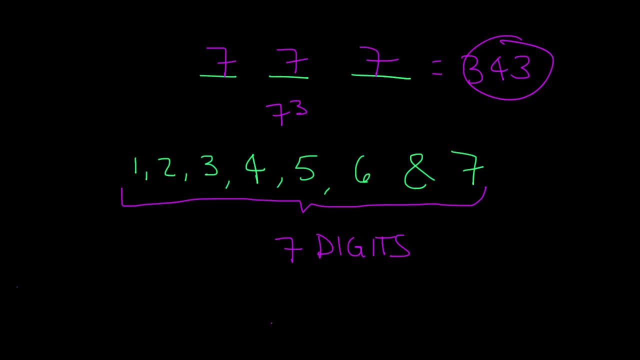 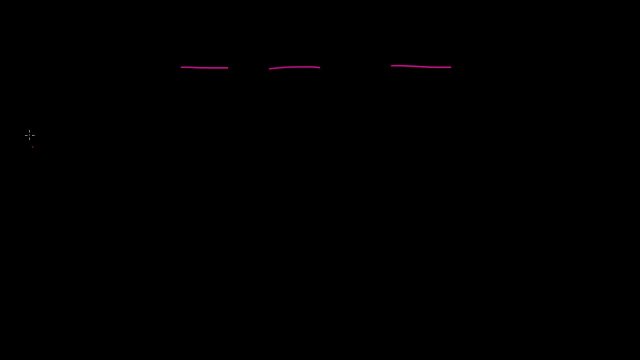 And from this word it can be made from six possible letters. So six letters, Six letters. these letters are F, G, H, I, J and K. okay, but repetition in the first one we're going to say is allowed. so repetition here is allowed. so if we go ahead and we 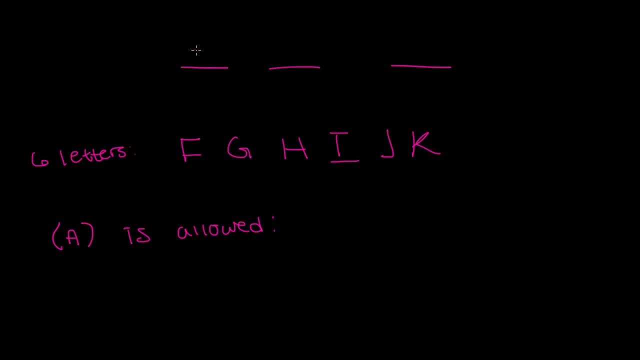 say, is allowed. there's six letters, three spaces, similar to the last problem. we would just say six here, six here, six here, and this would be six cubed, which equals two hundred and sixteen. easy okay. however, if we want to, whoops. if we want to have no repetition allowed, it's going to be slightly different, and the reason 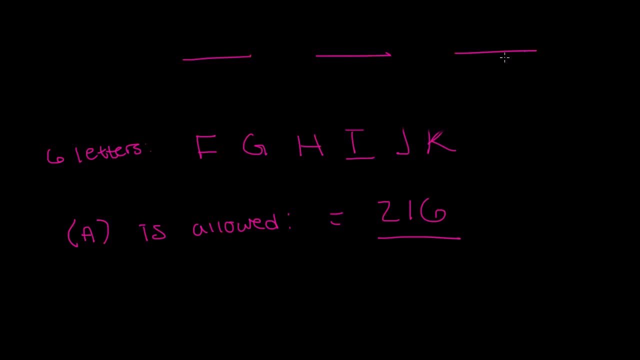 being is because okay, here, here, here, if we have six letters in the first one, then we've picked one of these letters. so now we're down to five possible choices. so the next one would have five possible choices, but then, since we have two letters picked from this standard set and then there's only